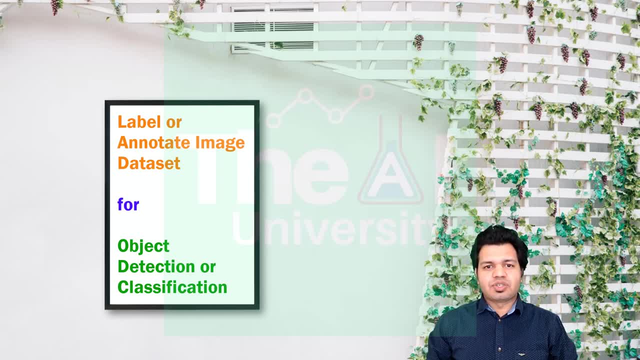 Do you know that in order to build and train any object detection model or classification model, be it using a standalone convolutional neural network or using YOLOv4 framework, you need to have image data set that is labeled or annotated? So how can you label your own image data set? 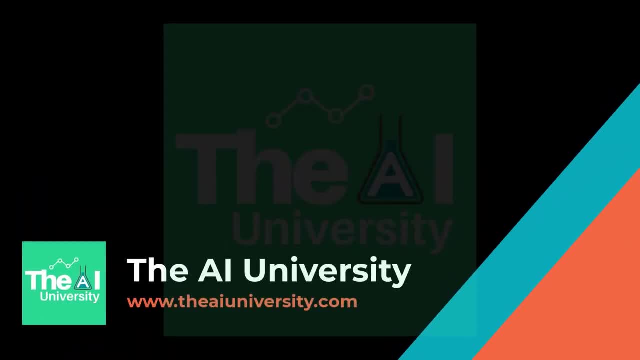 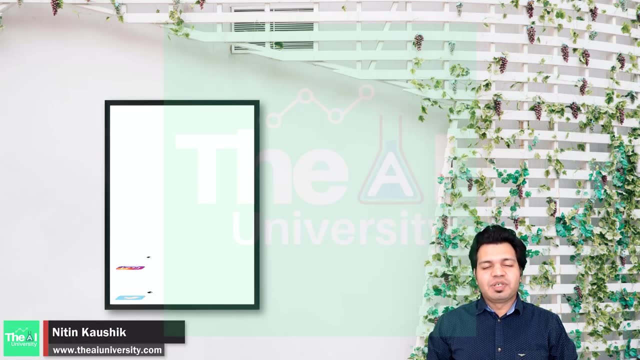 free of cost. Folks Nitin here, and this is the AI University channel. In this video, I'm going to tell you how to label your own image data set so that we can build our custom object detection model according to the data we have. For example, you may want to build an object detection model. 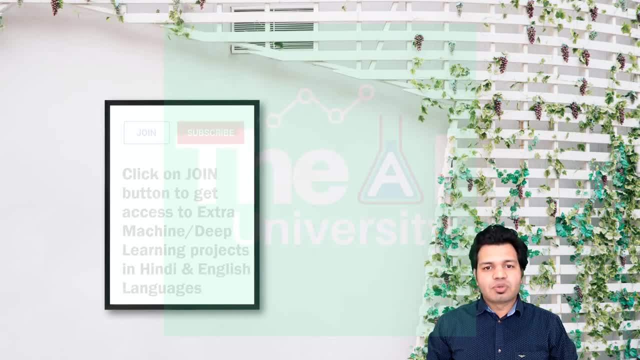 to detect home appliances. Somebody wants to build an object detection model to detect various vehicles such as cars, trucks, bikes, etc. So people might have different use cases. I'm going to tell you how to convert them into YOLO format so that these can be easily. 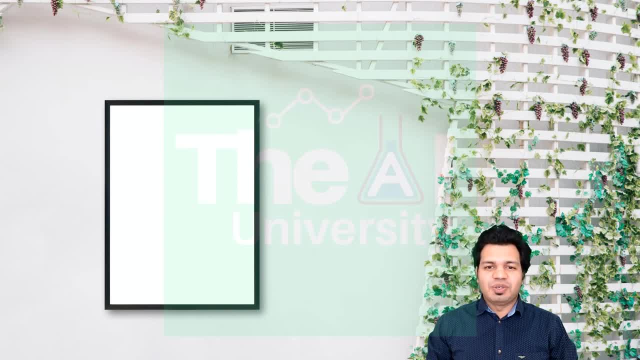 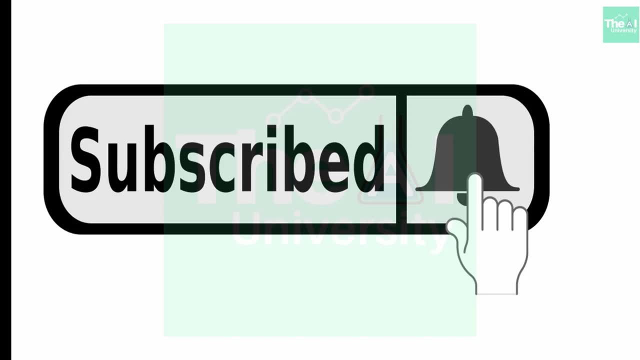 read during model training, So watch this video till the end. If you are new here, then consider subscribing to this channel. A lot of times I see people appreciating the content but forgetting to subscribe due to immense excitement. Please show your love and support. 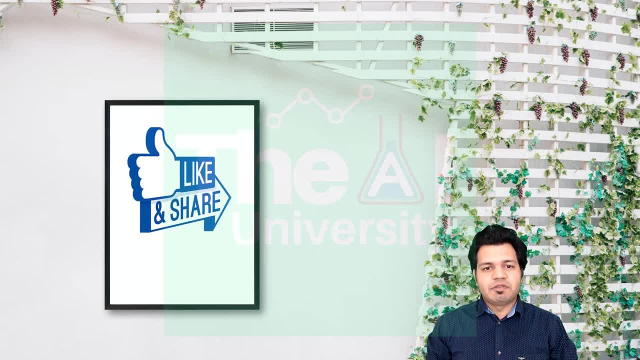 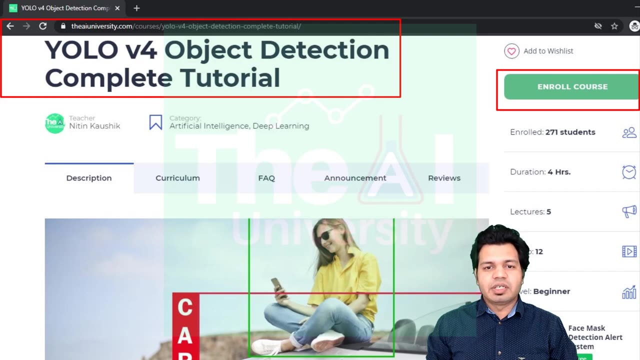 By liking, sharing and subscribing to this video, as I will feel highly motivated. If you have already subscribed, then click on the bell icon to receive the notifications about hottest technologies of 21st century. You can download the code related Jupyter Notebooks and other related material. 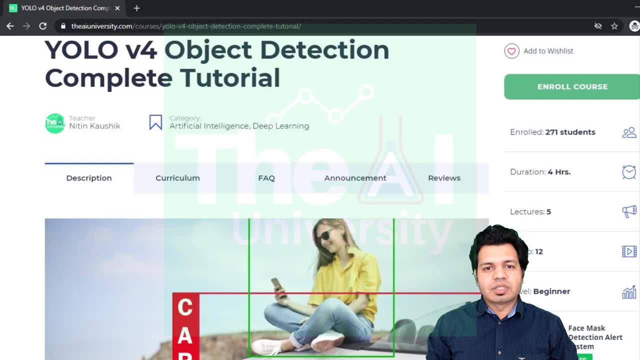 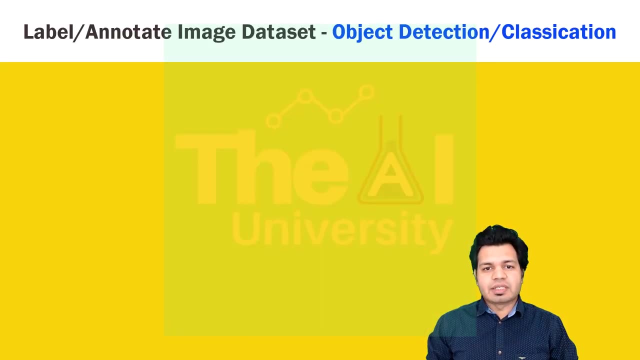 by enrolling to this course on the AI University website. If you like to go through these courses on mobile, then consider downloading the AI University Android app. The courses are offered free on our website, So you have your own image or video data set and wants to build your own object detection model. 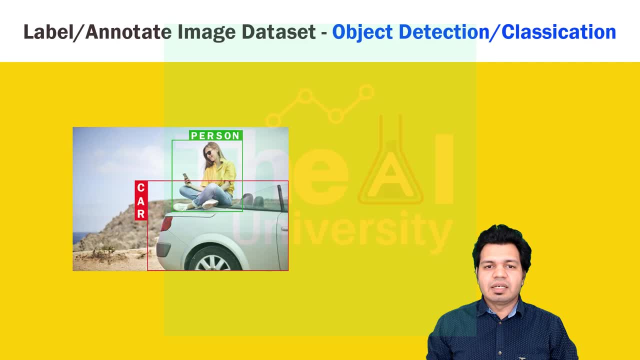 Image labeling or annotation is one and same thing and it means drawing bounding boxes around different objects in the given image. Bounding box labeling technique is one of the many annotation techniques and once we draw the bounding box, we then go ahead and label that object to identify. 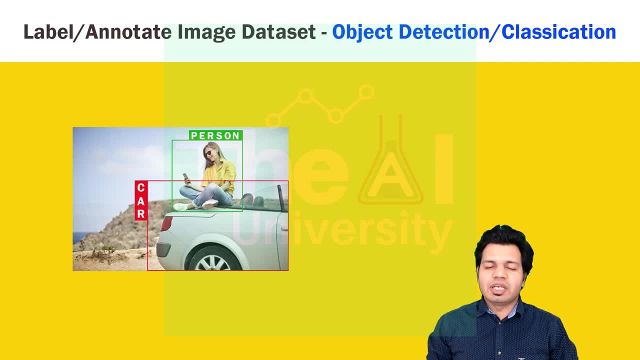 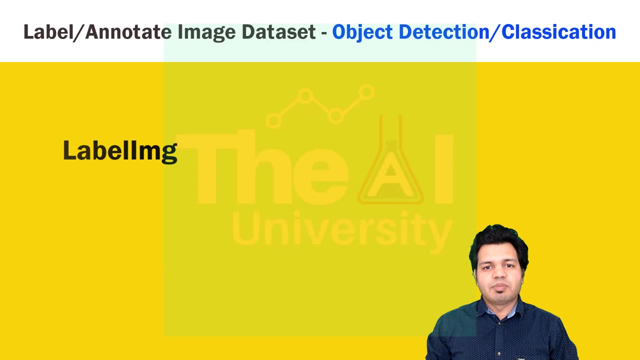 if it is a person, Laptop, bike or even a pet like dog or cat. Here we will be using a tool called as Label IMG, which is very simple to use and is free or open source, and which allows us to create bounding boxes. Using this tool, you can save your own. 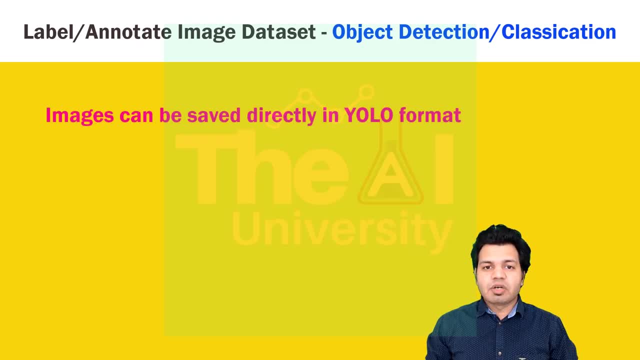 image directly in YOLO format. One of the good thing is that we don't need to resize any image in the data set and we can annotate images of any size. Yolo takes care of image size during training. Now let see how to install this Label IMG tool. 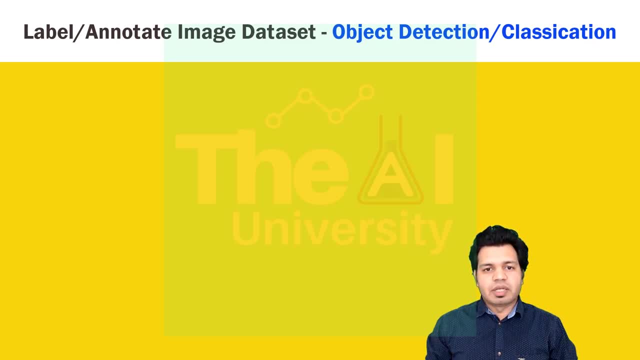 I am using Windows computer and anaconda distribution of Python, so I am going to show you the steps with respect to it only. But if, incase you have Mac OS or Ubuntu installed on your system, then you can just drop a message in the comment box and I will be. 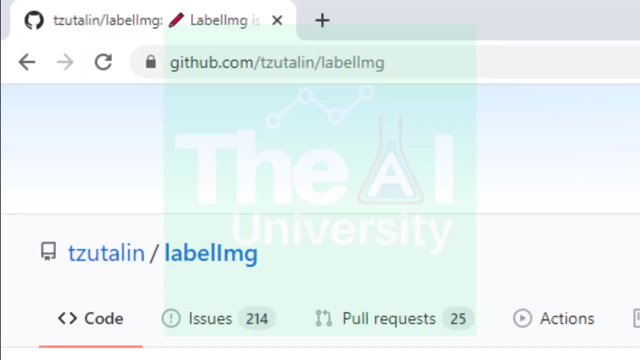 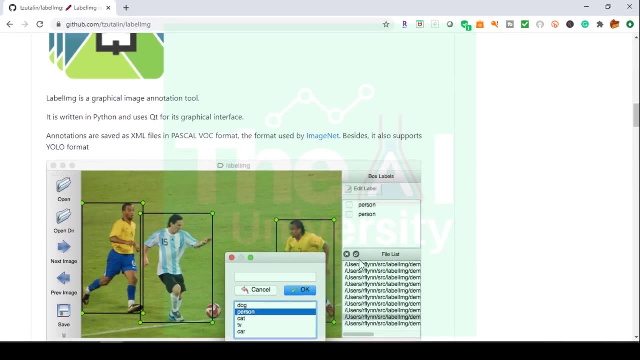 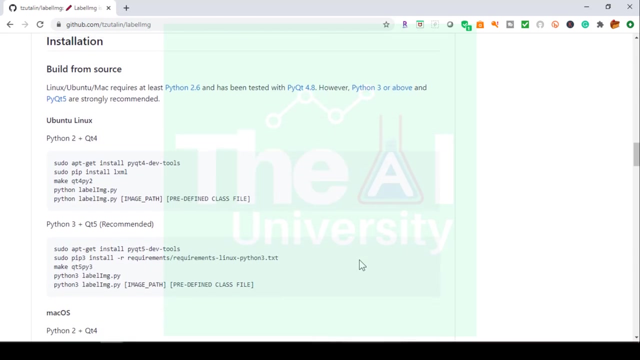 glad to share the steps for those as well. Here is the link to install the Label IMG tool. now let me scroll down a bit. okay, so they have given certain introduction and some documentation of this particular tool here. okay, and, as you can see, the installation steps are mentioned here and they have listed the steps for. 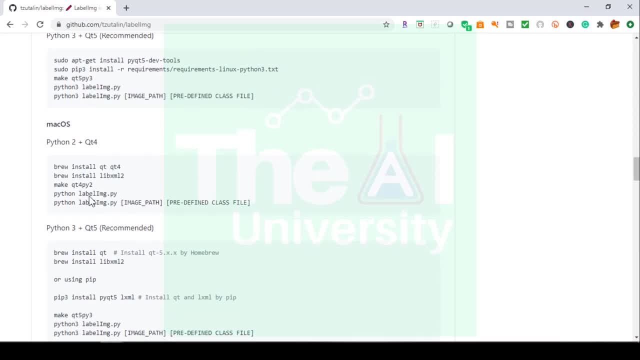 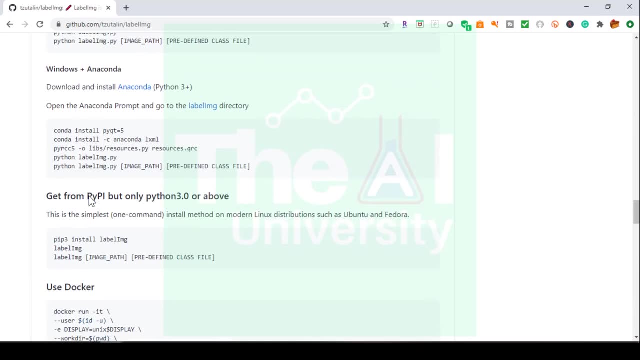 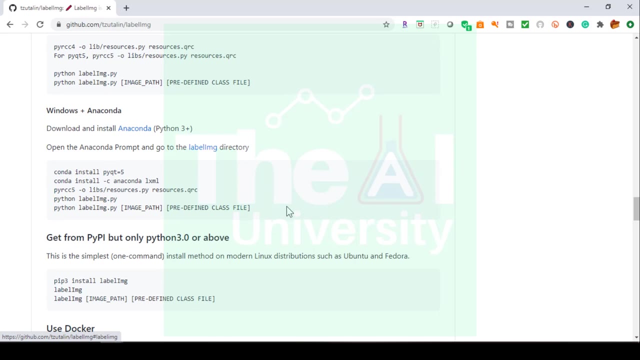 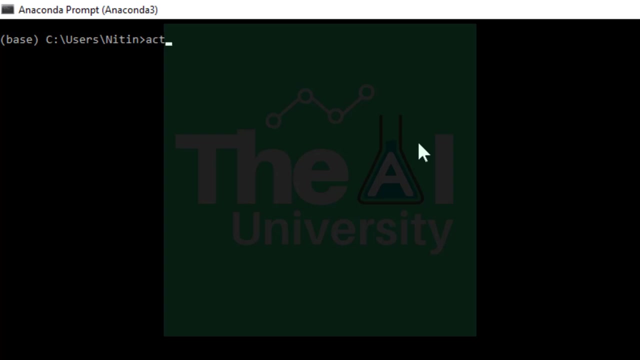 Ubuntu, Mac OS, Windows. right, this is, these are the Mac OS set of commands and windows, then windows plus anaconda and even docker. so I'm going to show you the steps with respect to windows plus anaconda only. so let me first open the anaconda prompt. so here you need to first activate your virtual environment. 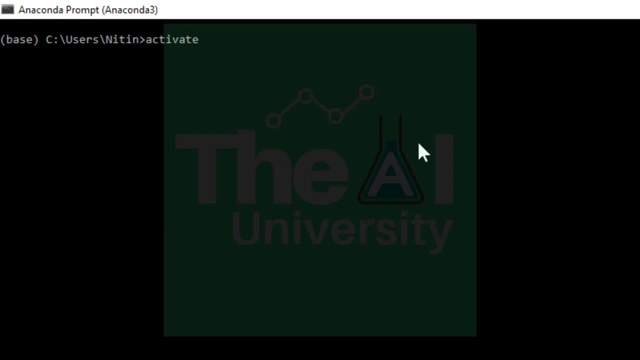 and the command to activate your own virtual environment is activate, and then the name of the virtual environment. I have already created one virtual environment with the name application env. hence I'm activating that environment only. so press enter so you can see that my virtual environment is activated now. now. 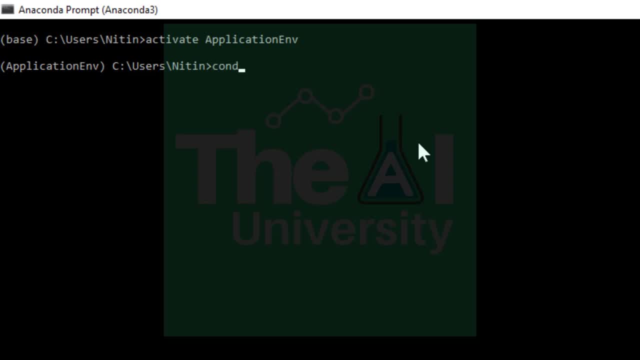 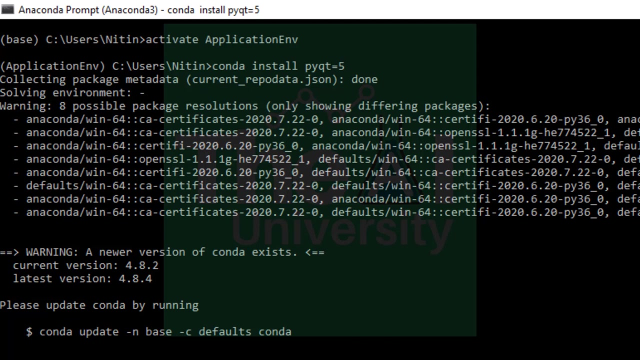 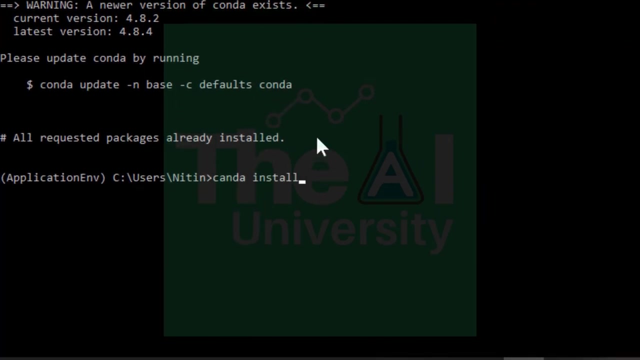 run this command, we need to install pyqt. so conda install pyqt equals to 5 and then press enter. so in my case this particular package is already installed. hence I'm seeing this message: all requested package package is already installed. now we need to install one more package, which is lxml, so you need to type conda install. 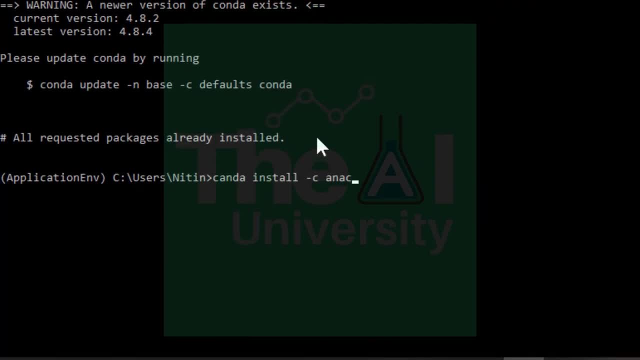 hyphen C, anaconda, and then lxml, and then fill in the command and the result will be remain same as what recipe, url, added code and so on, and you areatherine packages already. Och spor, then press- wait a minute, there is a typo, so it should be conda: install hyphen seek anaconda. 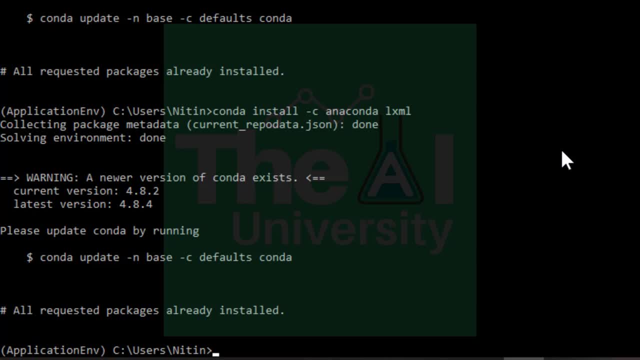 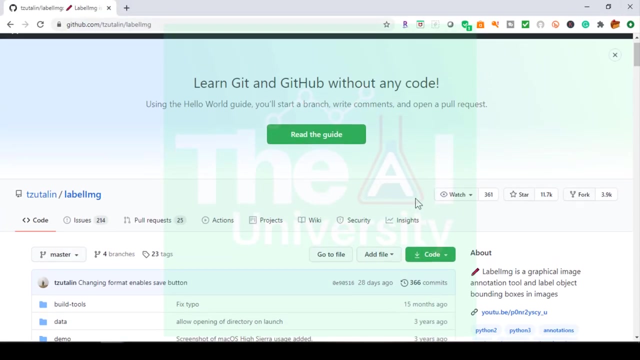 lxml and then press enter. so apparently this particular package is already installed on my computer as well. so now let's go to github page for label img and then download the label img tool from there, so as let's scroll up and you would be able to see this particular button, which is 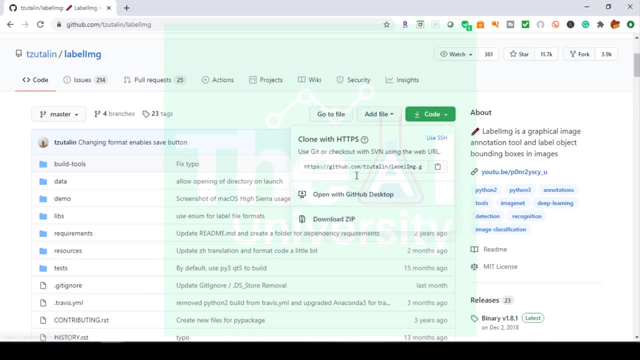 code. so just click on it and you will see a few options here. so just click on download- zip- and the download will start at the lower left corner. once downloaded, we need to unzip this folder and keep that folder in our c drives user location so you could see that i have first uh. 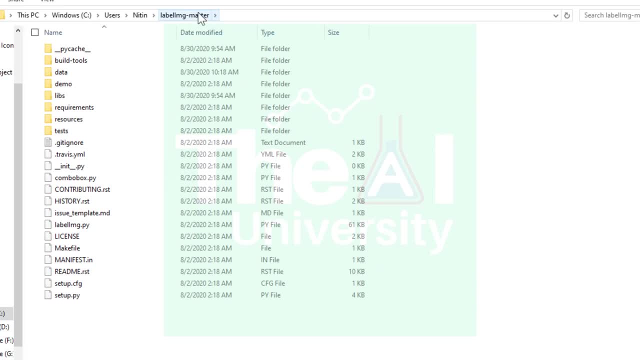 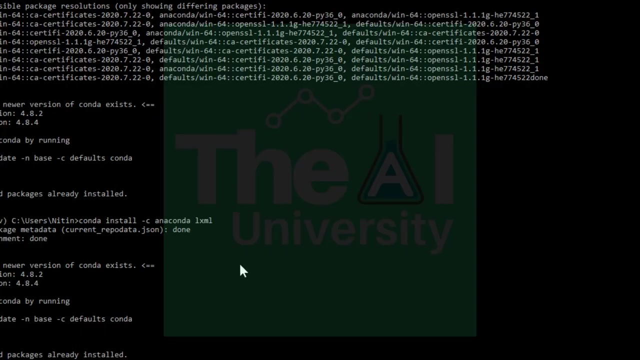 unzipped this folder, label img master, and then kept that folder or moved that folder into my c drives location, user location, right, and these are some of the files inside this particular folder. now let's go to the anaconda prompt and change the current directory to this particular directory, which is label img hyphen master. okay, so 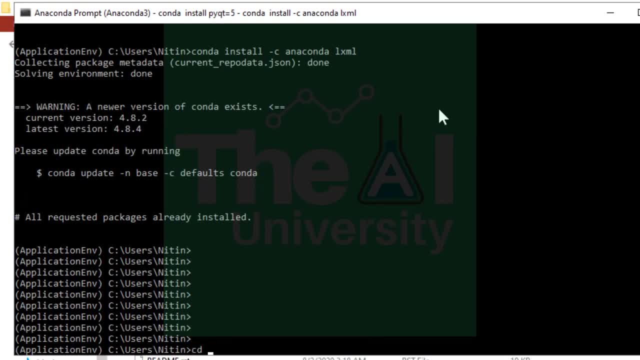 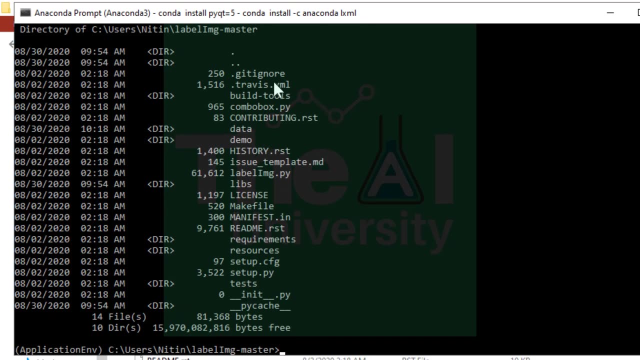 okay, so. so in order to go inside this particular folder, you need to type cd and then the name of the folder, which is label, img, hyphen, master. okay, when you type dir here, you would be able to see the same files. so dir is the windows command to see all the files, which is equivalent to ls command in. 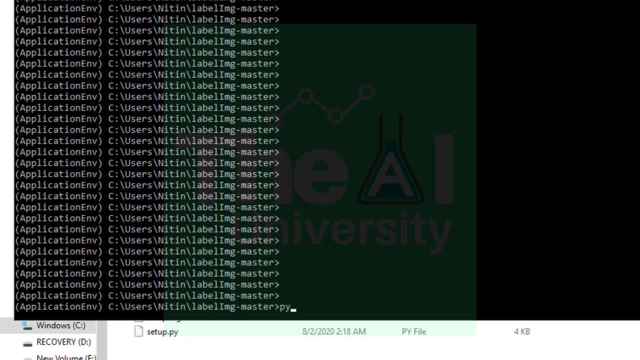 linux. so now run this command: pi r cc5 hyphen o, then resources dot py file and then the name of the file, resources dot qrc. okay, so this file, resources dot qrc, should already present in your label img hyphen master folder. okay, we need to have this file. 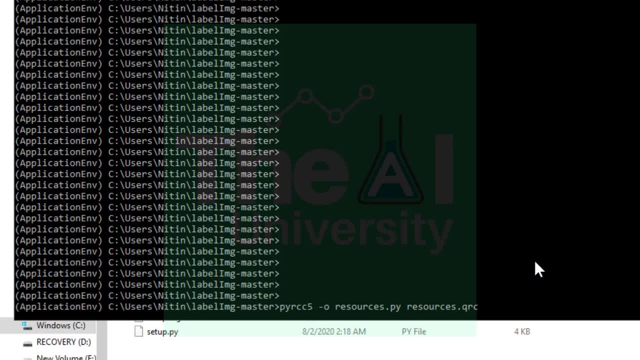 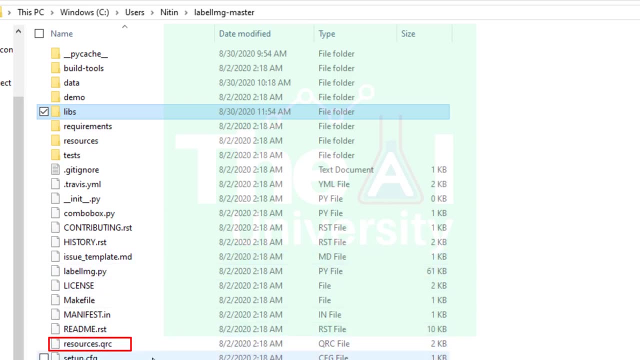 also created. so when we run this command, what will happen? uh, it will create this particular file as well, so resources dot py file in your label img folder. okay, so let me show you first one, so you can see that resourcesqrc file is already there. right press enter and you would. 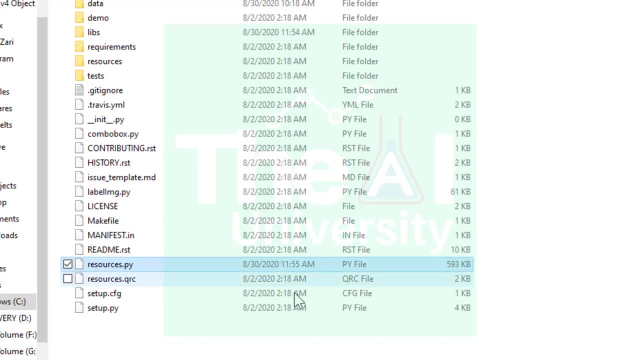 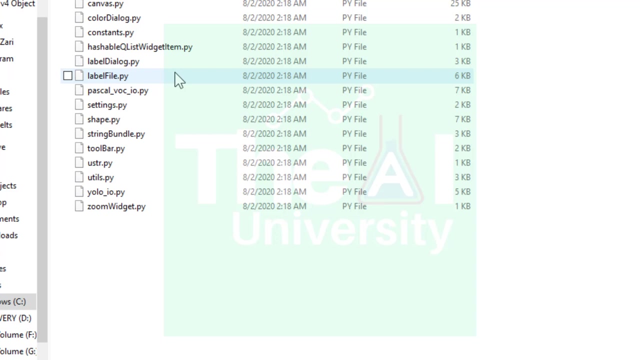 see resourcespy file, also created now. now you need to move these two files, resourcespy and resourcesqrc, inside this libs folder, so just cut and paste them inside this lives folder, this step, or copy these two files in the lips folder. then your chances are that. 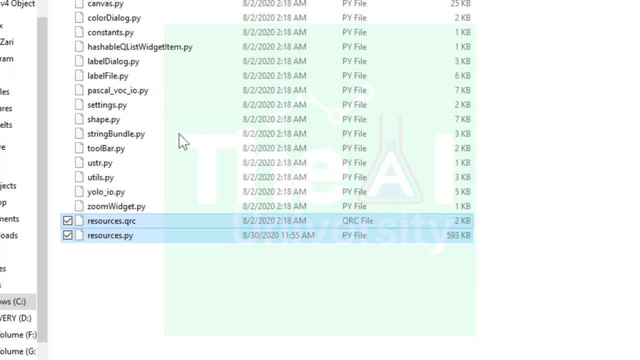 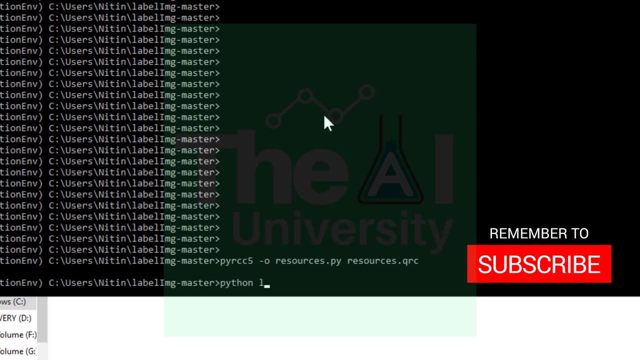 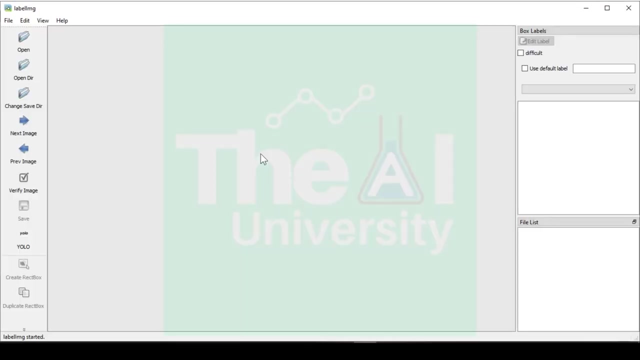 your installation is not successful. okay, once you do that, you need to run one command, now Python, then label IMG dot py, in order to initiate the label IMG tool or in order to open the label IMG tool. so press enter and then you will be able to see a window of label IMG, so just like shown here. so, using this particular 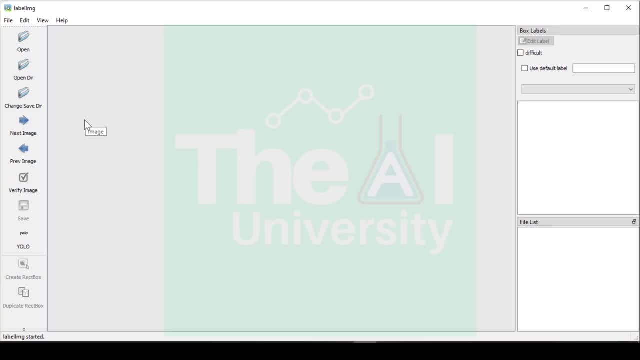 tool. I will show you how to label all the objects in the given image, so you can open any image by clicking on this open button and then browse to the location where you have kept your image that you want to annotate or label. so here is my image I have loaded into this label IMG tool now on the left hand side. 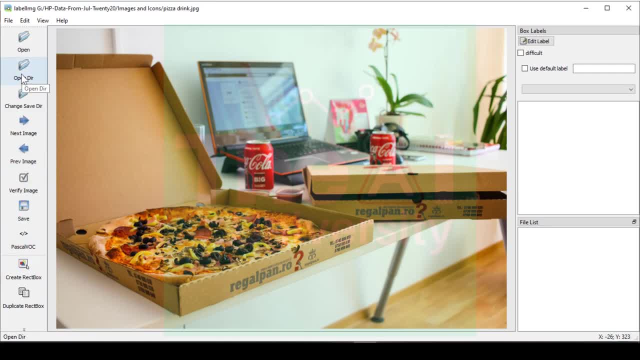 you would see various options here. there is one open dir button, so using this button you can open entire directory of images. then we have changed save dir button. this button is to basically change the directory to new directory where you want to keep your new annotated images. then you can use next. 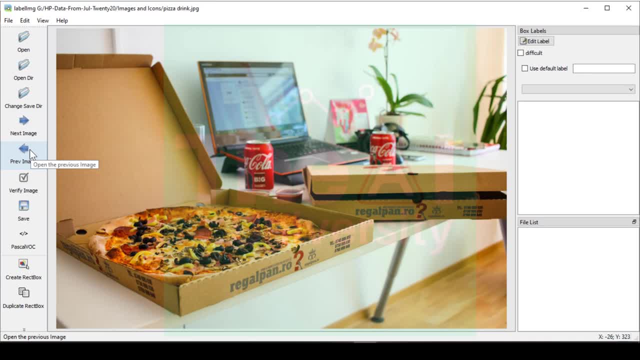 image and previous image buttons to scroll through images in a given folder. if you see down below, you will see these two downwards arrows. okay, just click on it and then you could see. you have options to zoom in, zoom out, fit to a button, fit to width button to clearly see the parts of the image to better. 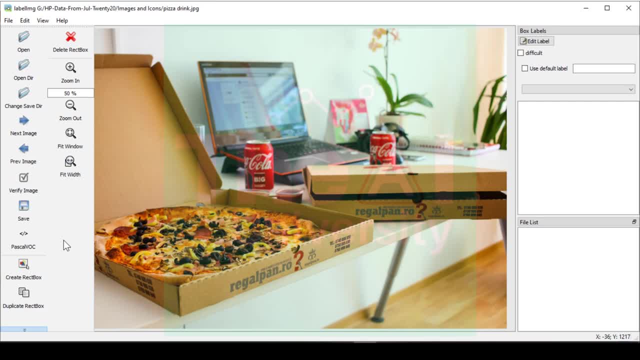 annotate them. so now let's label an object in a given image. okay, so just create a click on this, create a racked box button and then draw a bounding box around that. so you could see that I have drawn a rectangular box or bounding box around the object, which is pizza. you would see a pop-up window appeared on. 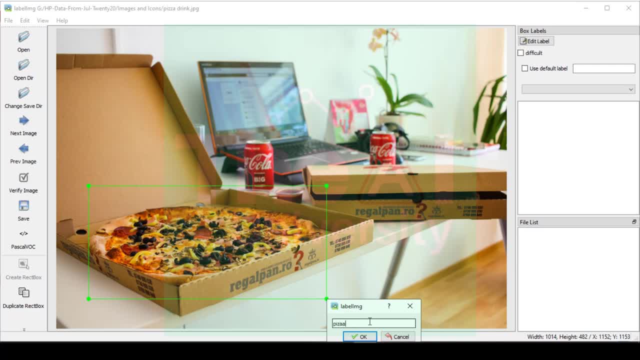 the screen. so just name it as pizza and then click on ok. so on the right hand side you would be able to see the label appearing okay inside this particular window right now. on the left hand side you could see that the format of this image currently is pascal slash foc. so just click on this button. 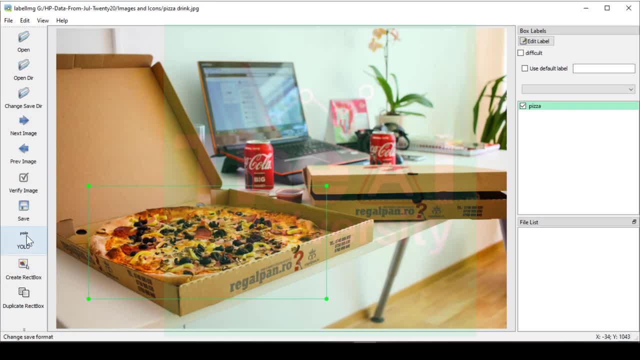 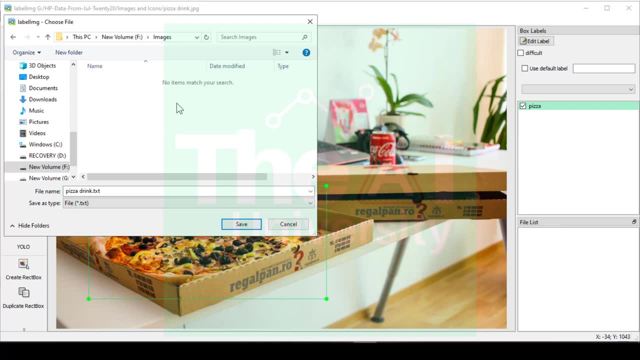 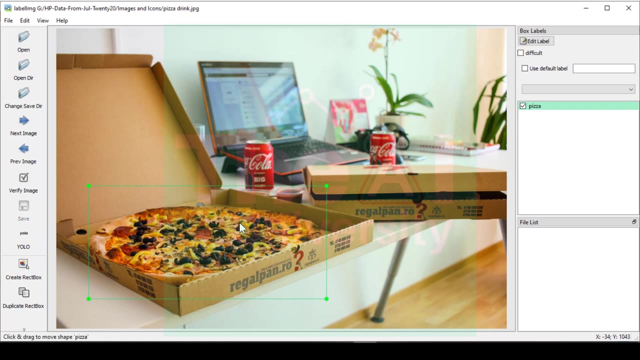 on the left hand side and change the format to yolo. so you can see that format is changed to yolo now and now you can click on save button and browse to the location where you want to save this, uh, these annotations. so click save. so as soon as you perform this operation, you would see two new 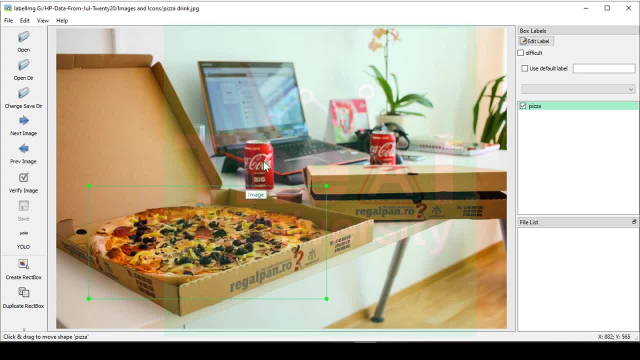 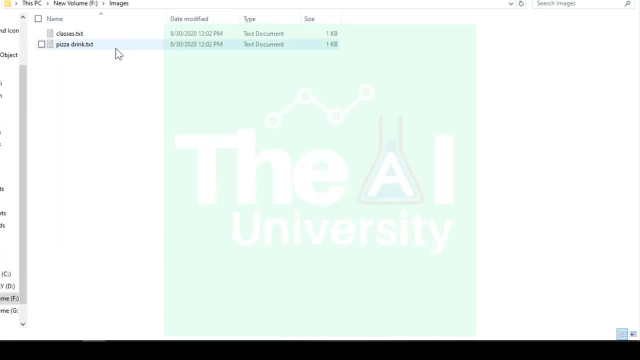 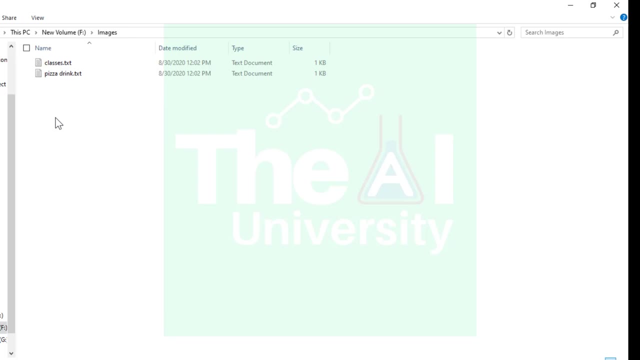 text files created inside the folder which i have selected from the browse button. so this was my location where i saved, uh, the annotations, and you could see these two new files created already now. the first file with the title classestxt, holds the class names or label names, and second file: 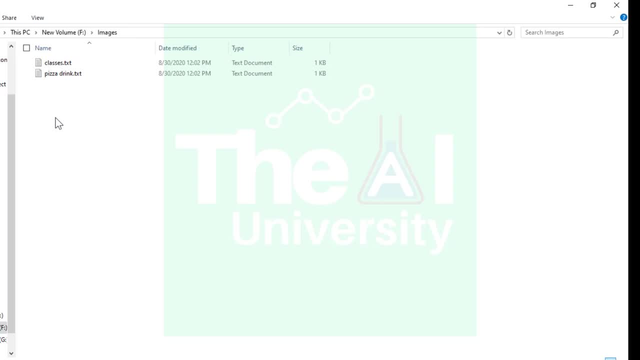 contains the annotated image in yolo format. let's open this classestxt file so you could see that with the name pizza is there in the classestxt file and that's the entry which we actually labeled in the image. now let's open this second file so it shows various numbers here. so first, 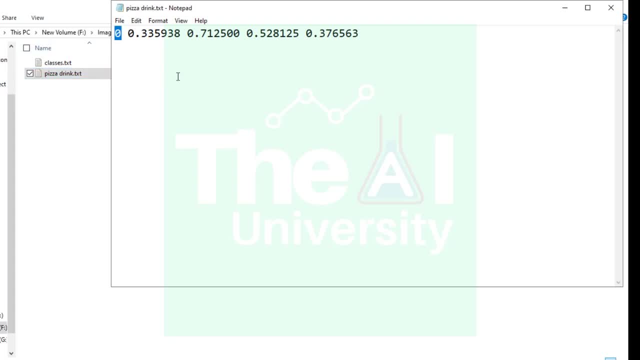 entry, which is this: zero entry suggests the location number of the class annotated, since pizza is the first entry in the classestxt file, so it is showing the number as zero because indexing starts from zero in this label img tool. next number is center point x of the 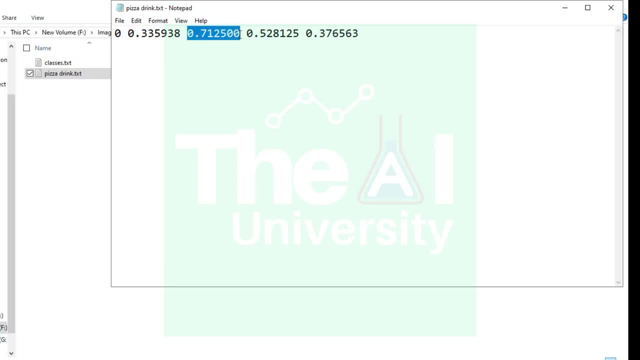 labeled object. next to it is the center point y, which is the point, center point y of the labeled object. next number is this object width and next to it is the object height. these entries, such as center x, center y, uh, width and height ranges from zero to zero, because indexing starts from zero in. 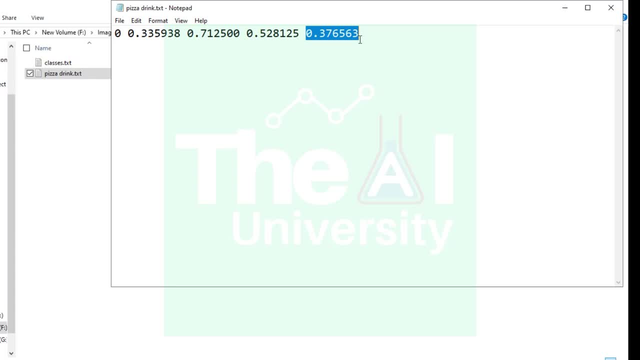 from zero to one. these values are normalized such that objects center- x value is divided by image width. objects center- y value is divided by image height. objects width: a value is divided by image width, and objects height value is divided by image height. now let's go back to the label img tool and try labeling few more objects. now let's. 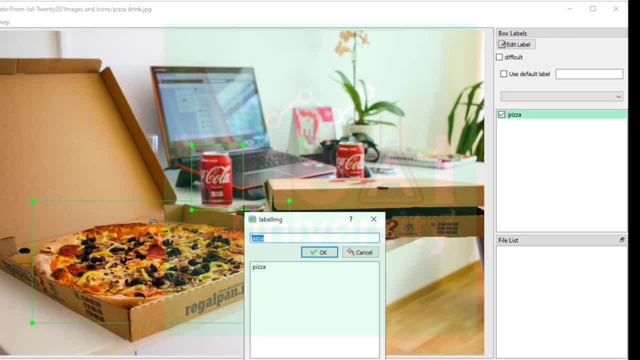 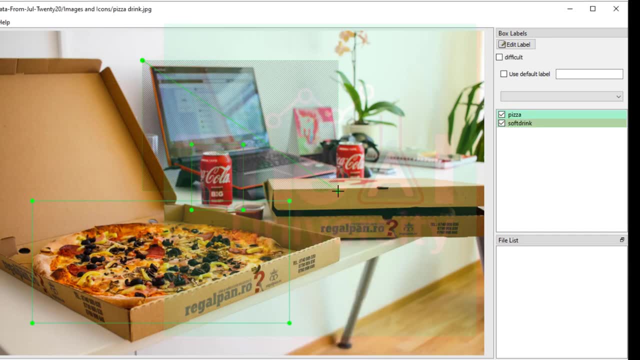 label this particular object and name it as soft ring, then label it as laptop. so you could see that i drew a rectangle of y bounding boxes around those two objects and label them as soft ring and laptop. now let's go back to our two txt files and see the entries there first. uh, we need to save them, okay, so save it. and then 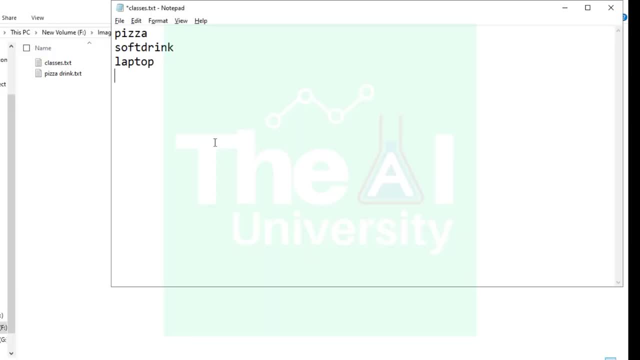 let's see those two files now, so you could see that as soon as i created those two new labels- soft ring and laptop, uh, there are two new entries in the classestxt file and two new entries in the pizza drinktxt file, and this is with respect to these two labels i have created, which were 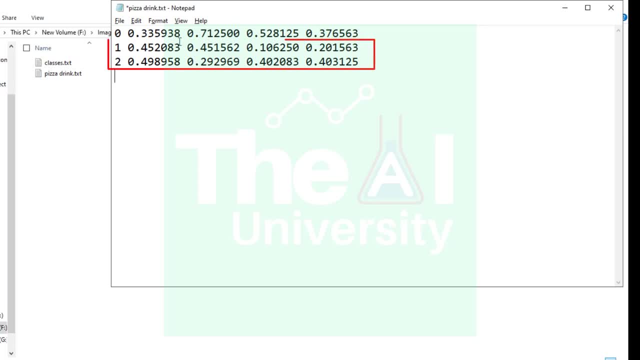 soft drink and laptop. so you could see that there are two separate entries for soft drink and laptop in two new rows and you could see the location number, center x, center y, width and height values for the soft drink and laptop entries. well, let's see. i want to change an existing label. 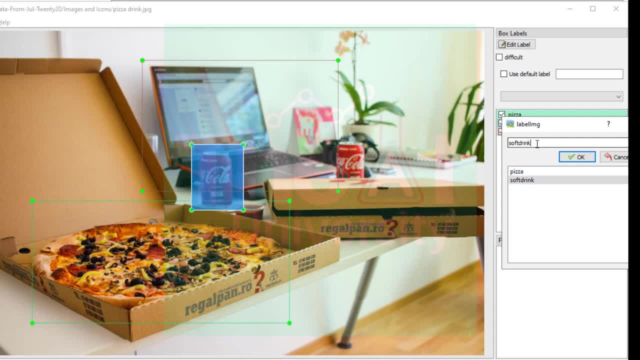 okay. so let's say, i want to change the label, uh, from soft drink to soda here. okay, so change the label and click ok. once you click ok, the label has been changed from soft drink to soda now. so you can do that and just click on save button. once you do that, a new. 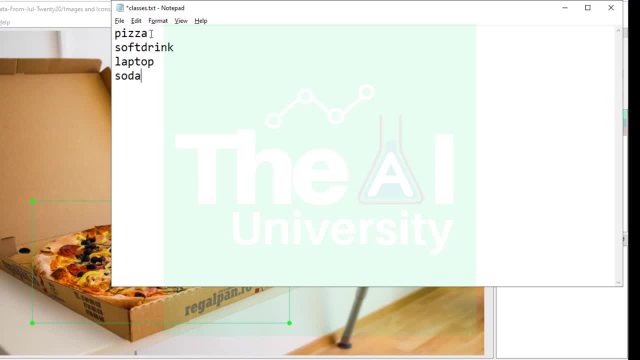 entry with the name soda will be created in the classestxt file at the location number three. so this is location number zero one, two and three. so a new entry will be created at the location number three for soda. now let's see the corresponding pizza drink dot txt file, which is our second text. 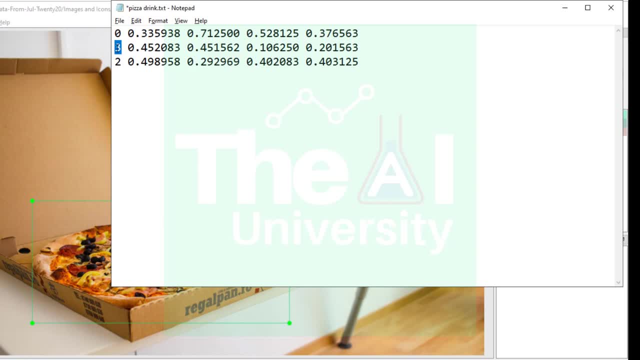 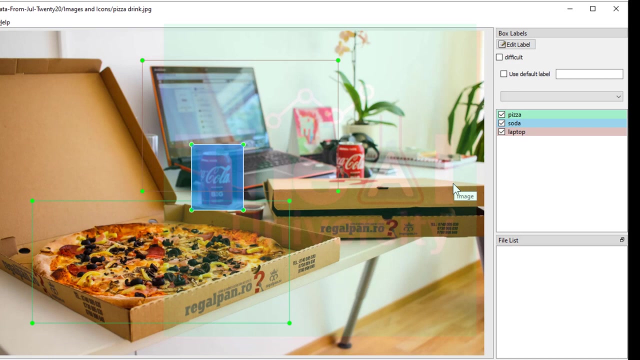 so you could see that the location number for soft drink has been changed from one to three. now, this is because we have corresponding entry for soda at location number three, rest. everything else will remain same, but just location will change. oh yes, one more uh thing. uh, in order to follow yolo format guidelines and standards, every image needs to have a corresponding. 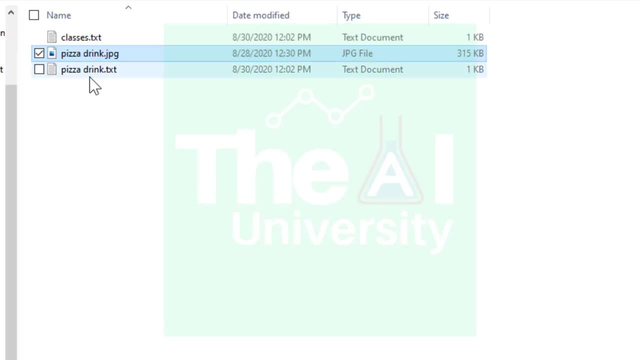 name same as our image file. so what am i talking about here is that our image name is pizza drink dot jpg, so we need to have the annotation file with the same name, which is pizza drink dot txt. so the title or name of these two files will remain the same, only the extension will change, and i'm 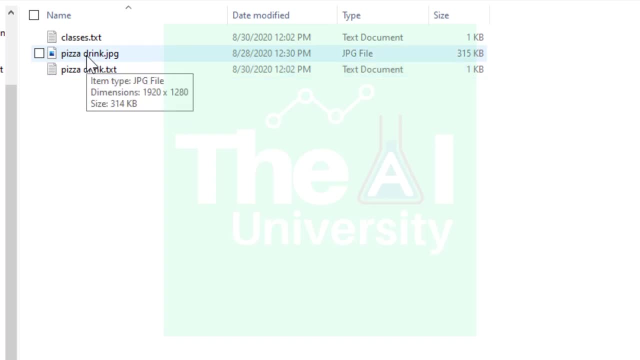 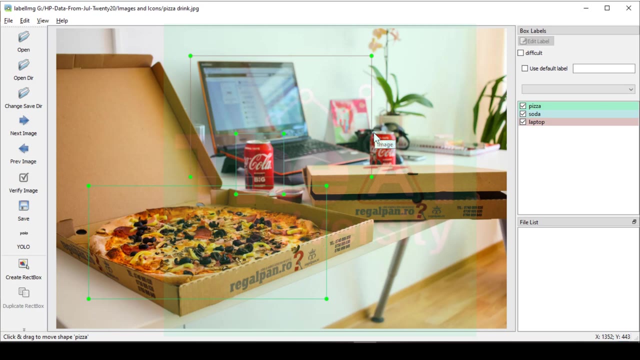 talking about annotation file and the original image file. now let's come back to the label img tool. so you can, uh, hide these bounding boxes. okay, and the way you can do it? you can just uncheck this, these labels, and the bounding box will disappear. so you can see that. bounding boxes for these three.